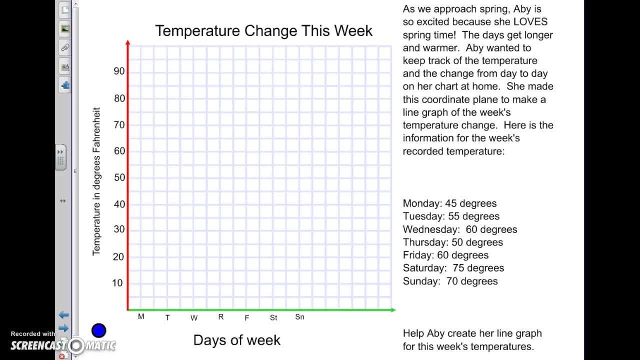 Tuesday: 55 degrees, Wednesday 60,, Thursday 50,, Friday 60,, Saturday: 75 degrees and Sunday it was 70 degrees. So quite a bit of change in that week, And what we want to do today is we want to help. 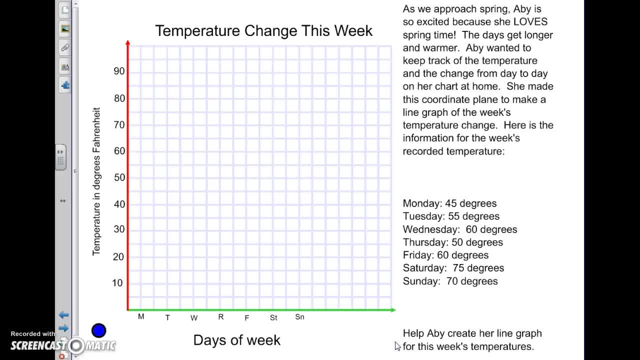 Abby create her line graph for this week's temperatures. So how are we going to do this? We are going to look. first of all, every graph should have a title, So the title for this one is temperature change this week. That tells us what when we look at this graph, when it's finished. 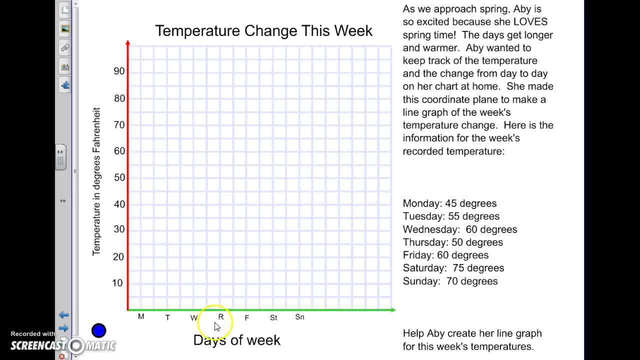 what it should be telling us. And then we're going to look at the x-axis, which, remember, is the one that goes side to side and that's telling us the days of the week. So we've got here and there's one here that's a little bit different, that you might be wondering about. 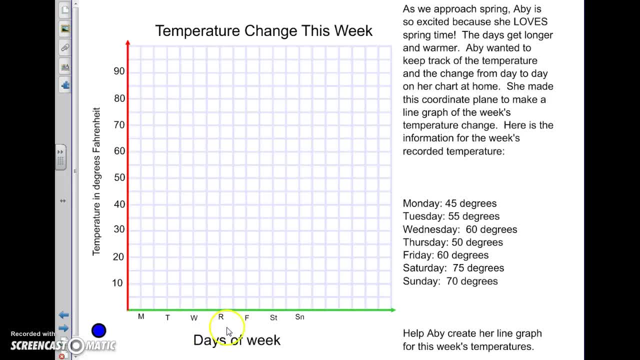 so I'm going to tell you. So the m is obviously Monday, t is Tuesday, w is when, r is Thursday, f is Friday, Saturday is st and sn is Sunday. And then on the y-axis here going up is temperature in degrees Fahrenheit, So you can see that every two lines up is 10 degrees. 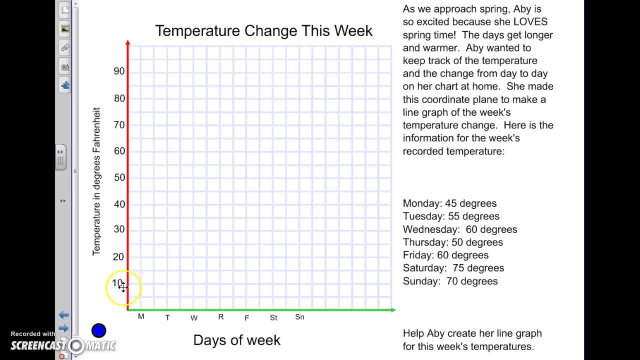 So we start at the point of origin: 0,. 0, go up 10.. So obviously each one in between is a multiple of five. So we've got 5,, 10,, 15,, 20, and so on all the way up. 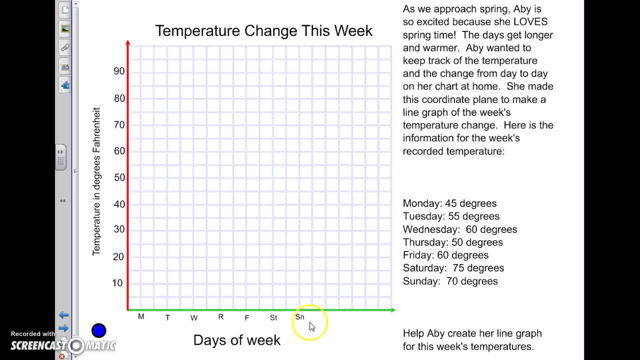 we've got 90 here marked and then for the x-axis, the days. just for spacing wise, so it's not quite so crunched together, I space them out to two different lines in between. okay, all right, so we see here that on Monday it's 45 degrees. so to mark that obviously we're going to go on the x-axis to. 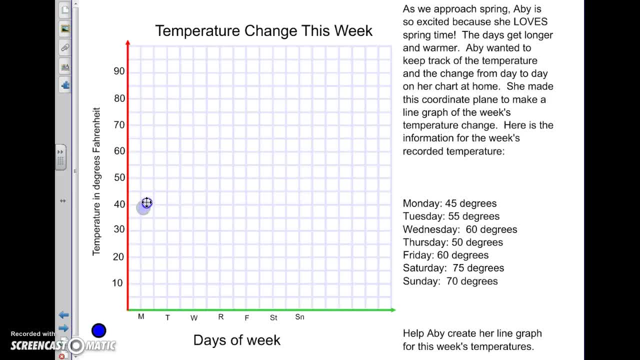 Monday, and then we're going to go up to where we see 45 degrees, so here's 40, here's 50. remember, each of these lines is a multiple of five, so 45 degrees would be right there. Tuesday is 55, so go to Tuesday, we're.